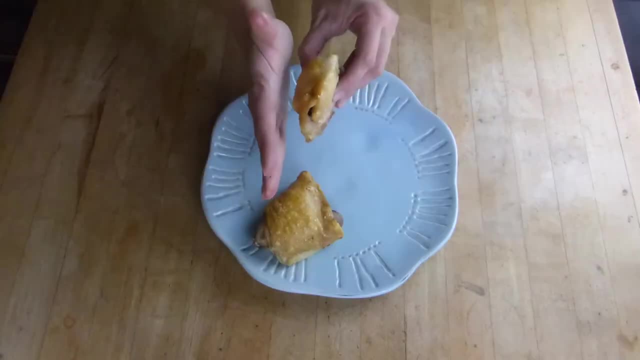 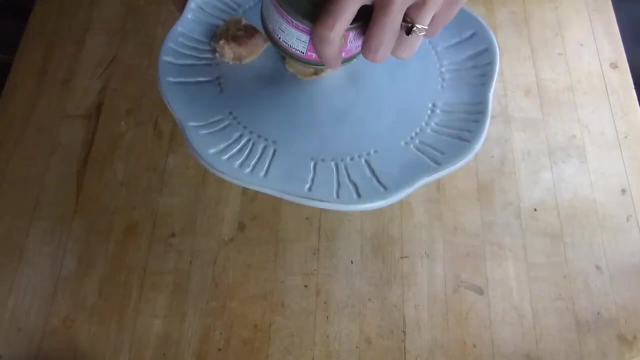 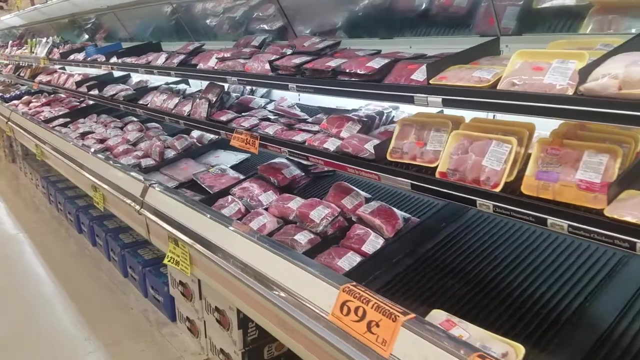 start out with measuring protein sources. for that we're going to use the palm of your hand. i would recommend having one or two servings of protein with each meal, where a serving is the size of the palm of your hand. now, to be clear, i'm talking about foods that are primarily protein. 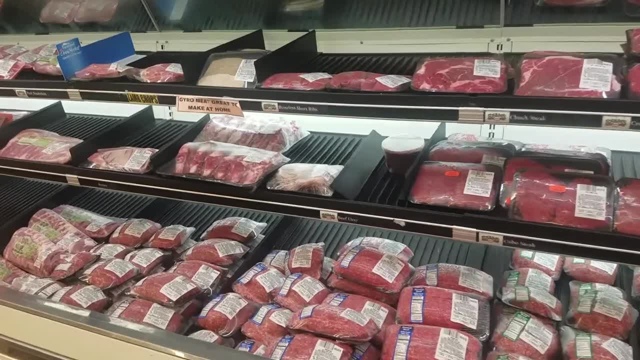 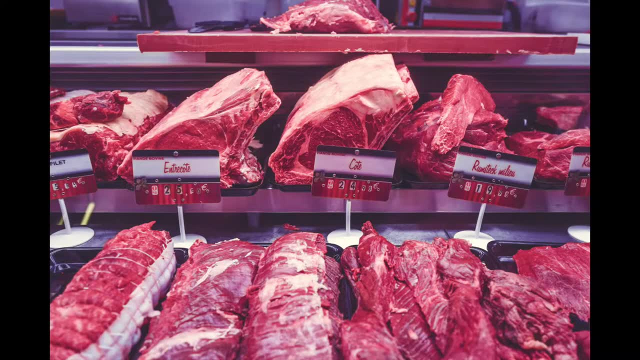 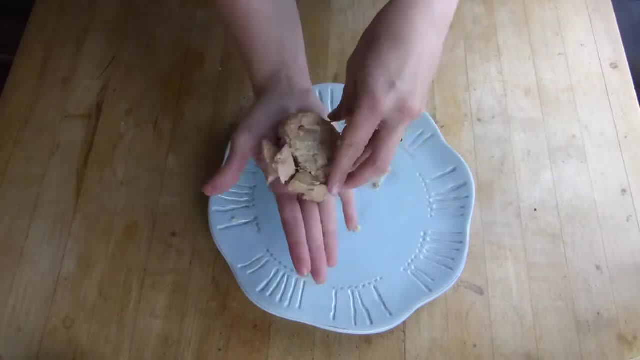 so this wouldn't include things like lentils or beans, which we would actually classify more as a carbohydrate. so just to keep things simple, let's specifically focus on meats like chicken, beef, pork or fish. eye out the size of the cooked meat based on the diameter and width of your palm. 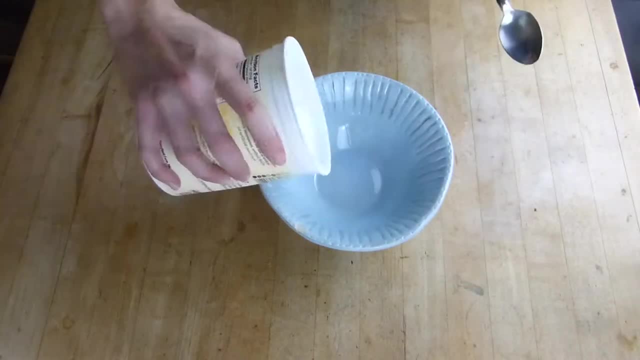 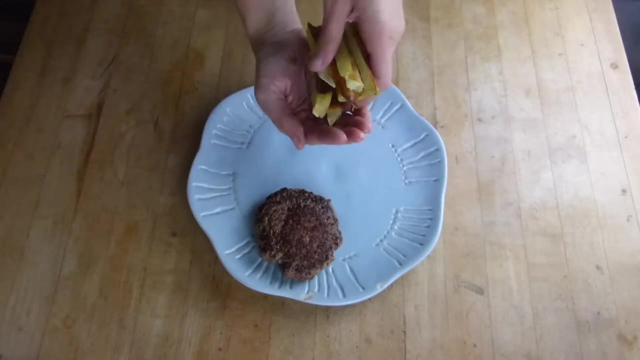 and actually here i'm going to include dairy products like yogurt, but only if it's yogurt not packed with extra sugar, which you'll want to watch out for big time. next would be your starch or carbohydrate, which you can measure by cupping your hand. so if this is rice, it would be a cupped handful of cooked rice, or if it's sweet potato, a cupped. 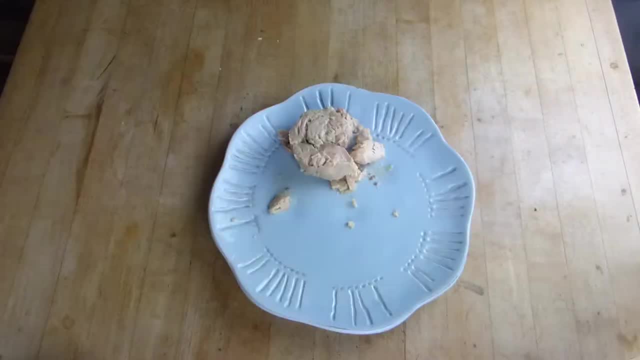 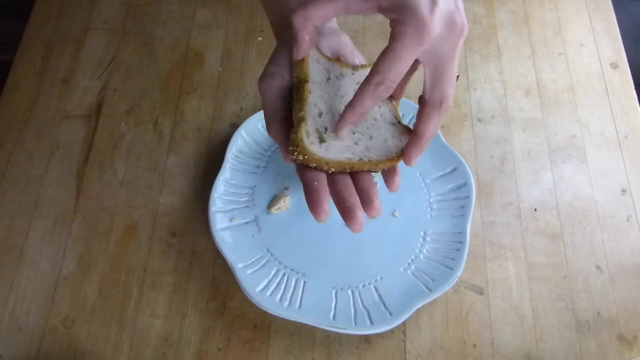 handful of cooked sweet potato. if it's bread, and then i know this one is tricky, but do your best to eye out a handful of bread. i'm not saying you have to squish your bread into a ball, but keep in mind that as you go through this and do this more often, it's going to become. 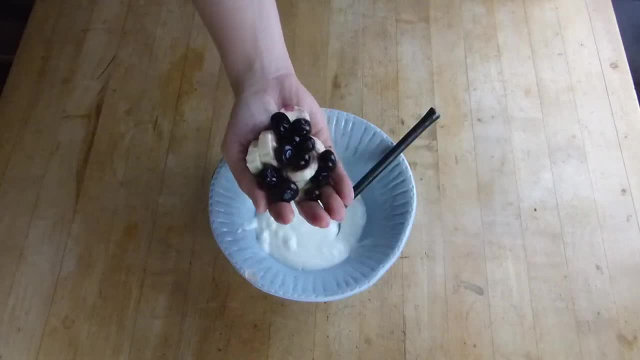 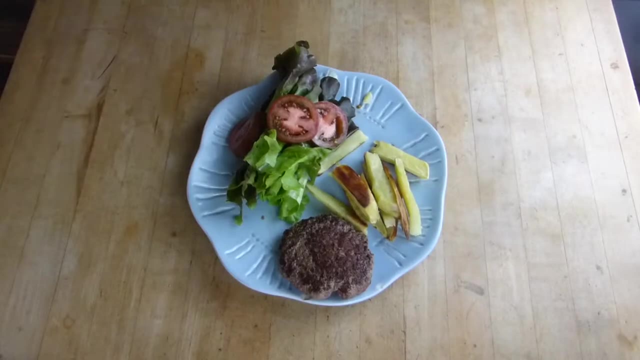 easier to eyeball out that portion size really to your hand. fruit would be included in here too, so you can measure, say, a cupped handful of bananas or berries. you get the idea. now let's look at fats, which you can measure using the size of your thumb. 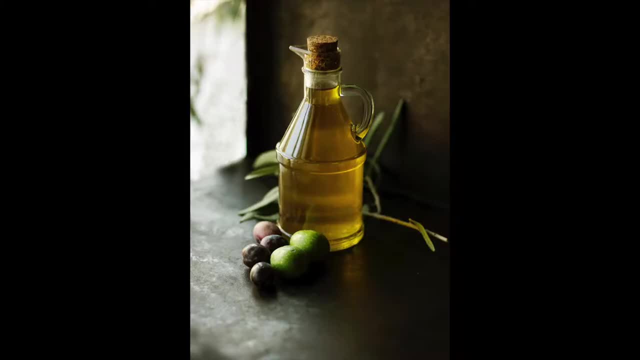 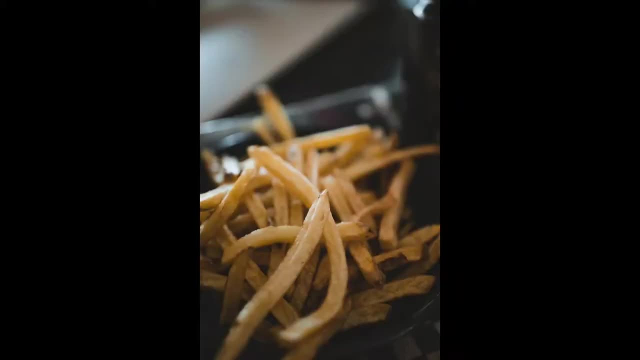 so the length and the width of your thumb. people often go way overboard with cooking oil and it's one of those things in eating meals out that is like a hidden calorie. since you can't see it, you can't see the oil, you don't know how much was used if you didn't do the 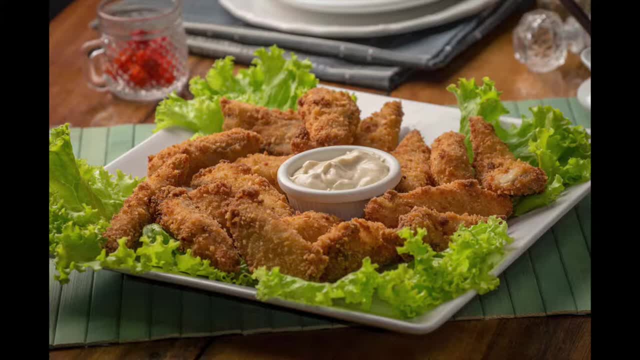 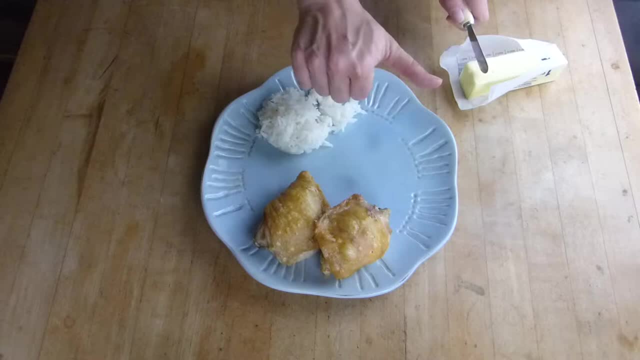 cooking yourself, so that's why it's always way easier to eat at home when you've done the cooking yourself and you know exactly what's in your food. if this is cooking oil like ghee, coconut oil or something else- liquid, i know this can be tricky, but just do your best. 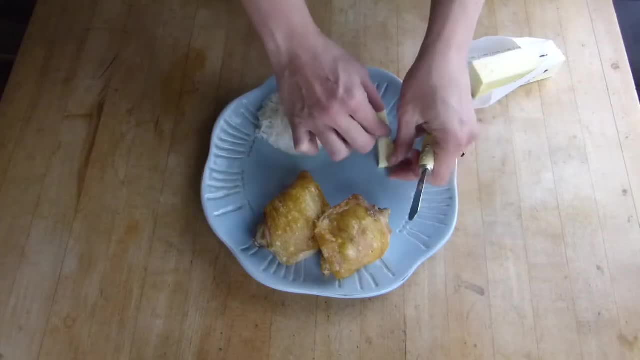 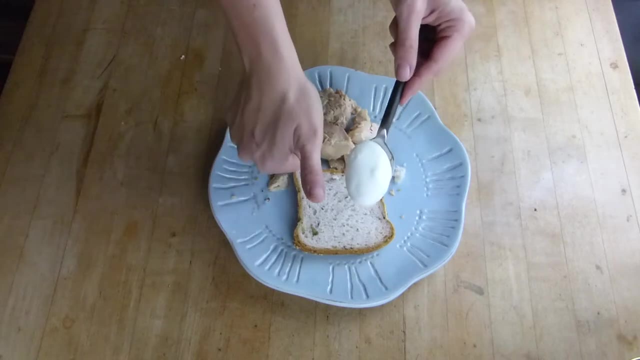 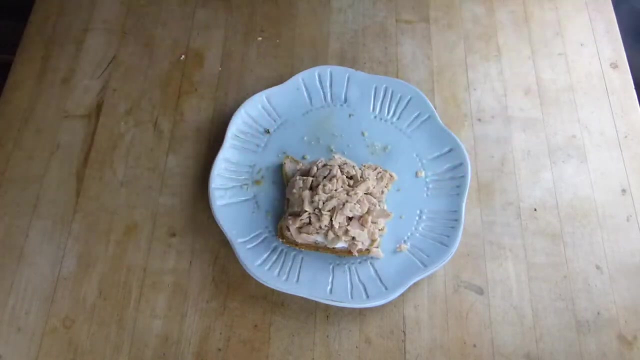 maybe even use a spoon to measure it out first so that you can get in, get a better eye on it. if this is a condiment like mayonnaise, same thing here. cheese, just side note here, because cheese is kind of a fat but it's also really high in protein. 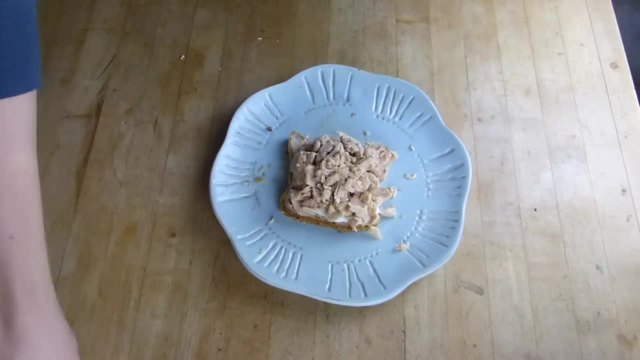 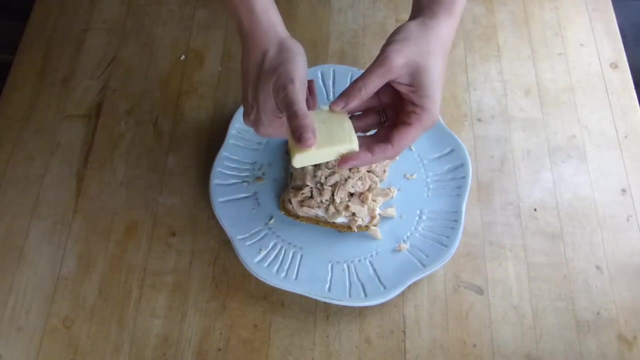 it kind of straddles that that line between the two. i would go a little heavier on cheese, especially if it's like lower calorie cheese, like mozzarella or that kind of thing. so for cheese, maybe two to three thumbs full again, since this is a lot of protein and it has a dual purpose. 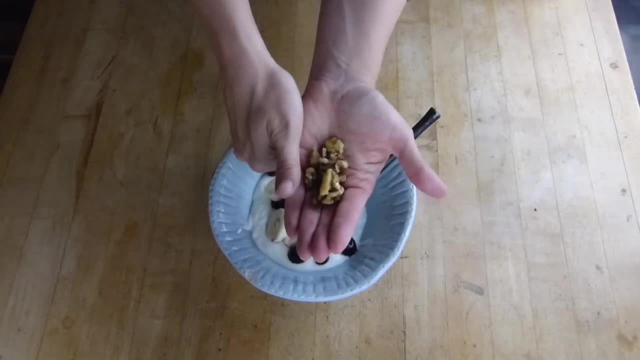 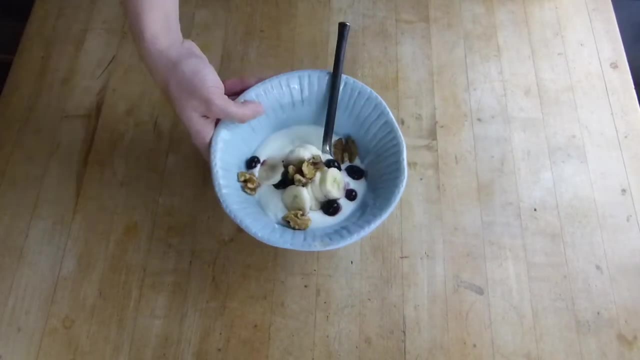 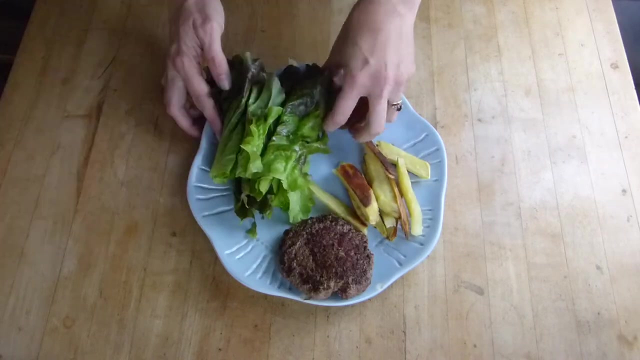 peanut butter or nuts- again, the size of your thumb. that covers your three primary macronutrients: protein, carbohydrates and fats. and the other category i want to include here is vegetables. you want to shoot for one to two portions of veggies at all of your major meals. 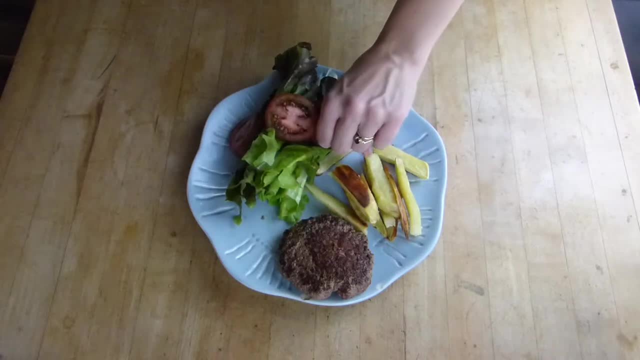 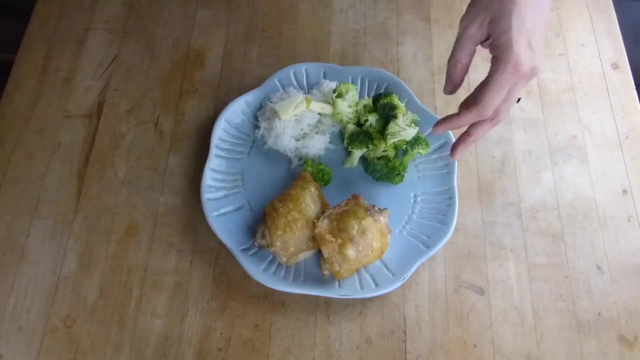 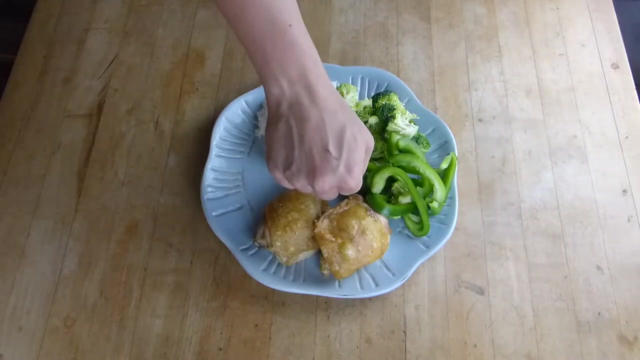 which we will measure using your fist. so a fist's amount of lettuce and tomato, a fist's amount of carrots, a fist's amount of broccoli and or bell peppers, and we'll go ahead and do that and leave veggies out of your yogurt bowl. thank you very much. 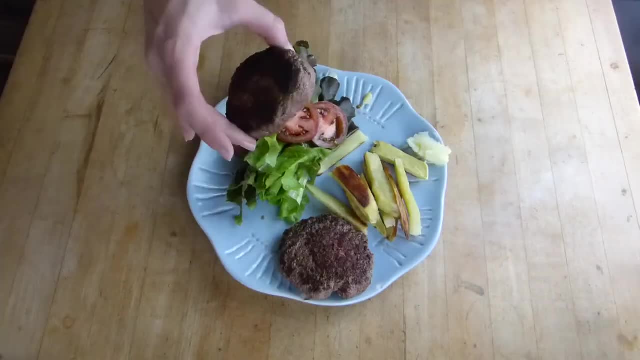 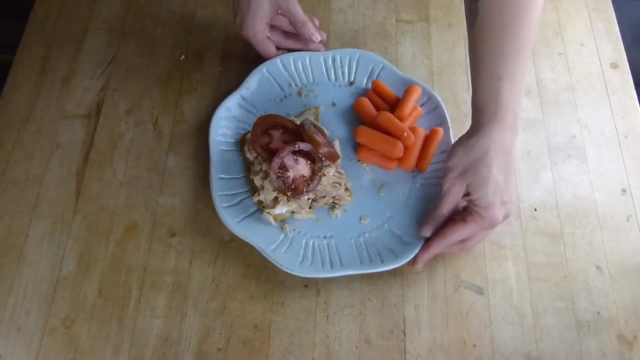 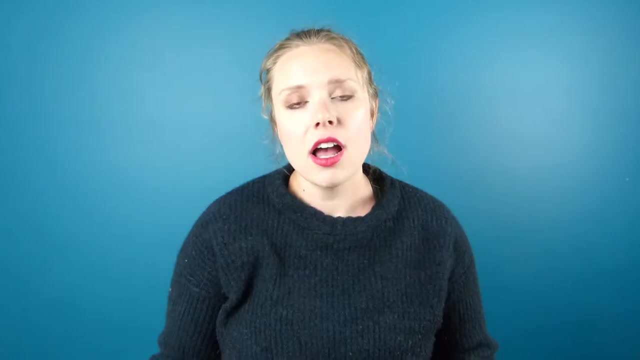 and there you go, you've made your meal and it's perfect for you. we have one to two portions of protein, a portion of starch or carbs, a portion of fat and a couple portions of veggies. now, you might notice that i didn't include here odd sorts of snacky foods like 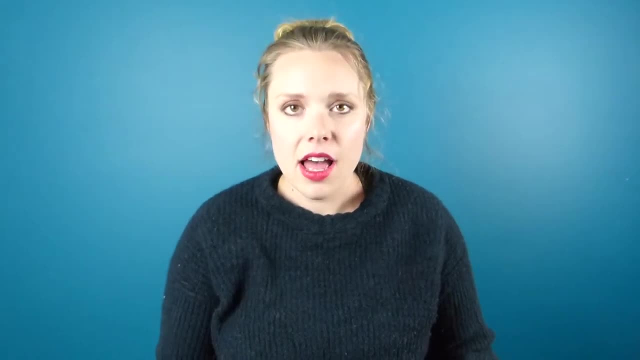 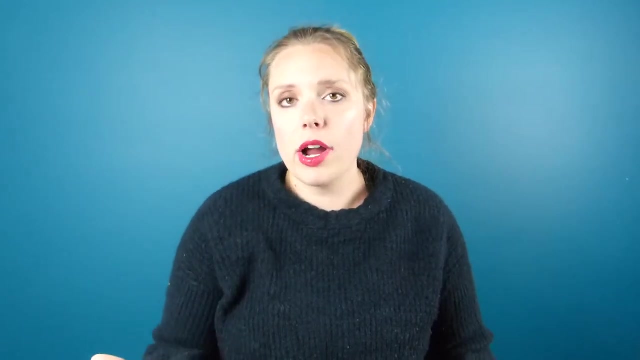 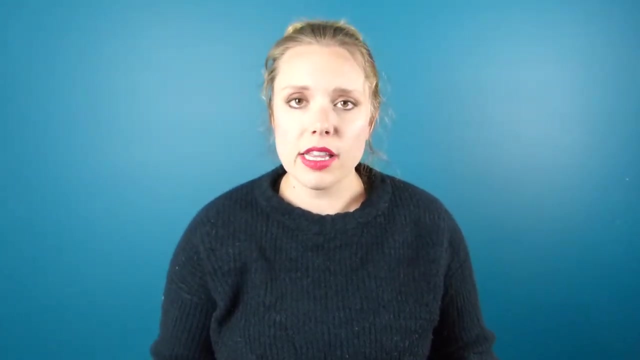 chips, candy, you know that sort of thing that doesn't exactly fall into like one of those categories, and that's just something for you to be aware of. maybe, uh, eating moderately while you're trying to lose weight because, remember, if your goal is weight loss, um, you really want to try to stick to nutrient-dense whole foods. 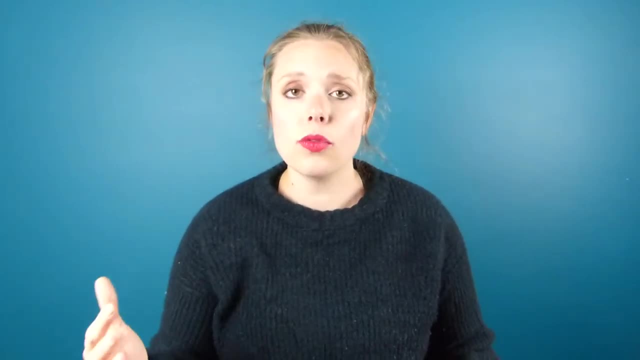 and what i mean by that is, everything we've just seen here is a whole food, meaning it hasn't really been processed a lot, um, it's kind of in its whole form, so whether that's dairy or meat or rice, that kind of thing. so i like to recommend at least starting off with these. 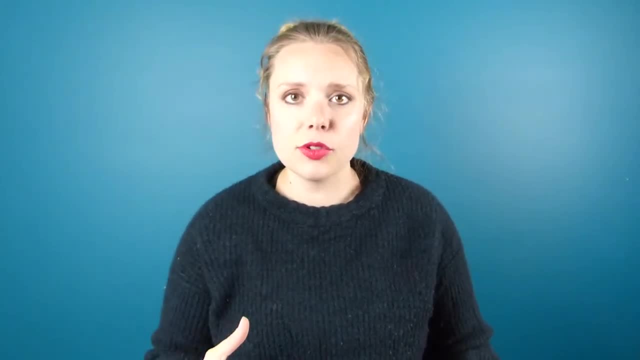 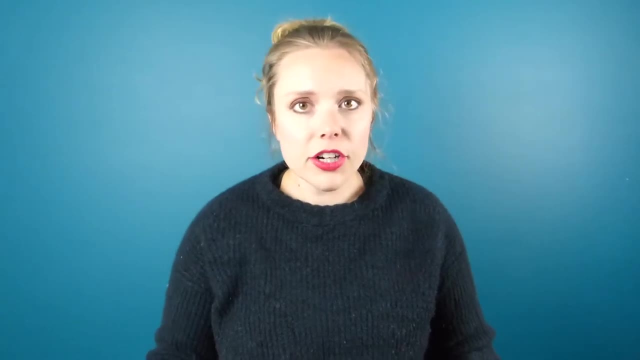 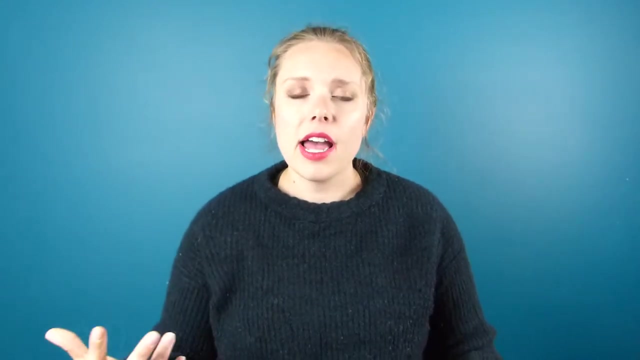 nutrient-dense foods, building your meals based on these foods- whole foods- and get used to what that looks like and then afterwards, if you're still hungry or if you need a snack, then you can kind of build in these, uh, more processed foods like in here and there again, just kind of being mindful. 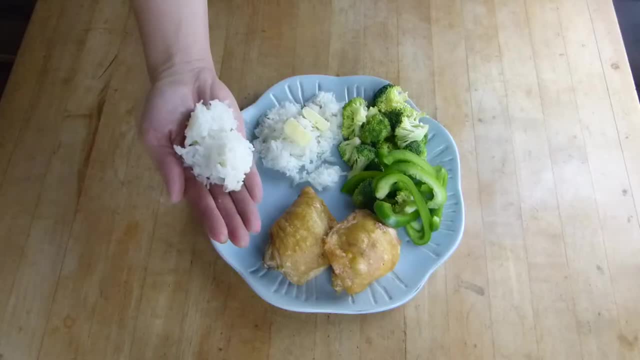 of what place they have in your weight loss program. what's cool about this process is that if you want to eat fewer carbs and higher fat, or vice versa, you can simply swap out. so if you want to eat a little extra carbohydrates, just take away a little bit of the fats. now you're also going to notice here that 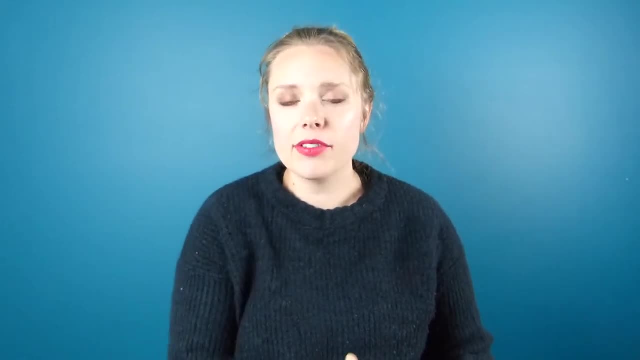 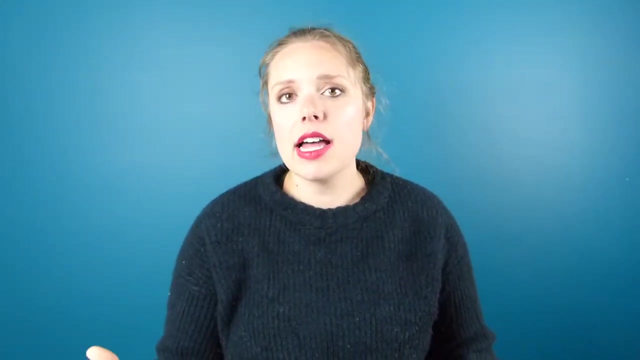 hillary, like some of these meats that you're portioning out are like, have hugely different caloric uh values. yes, so tuna, fish or chicken breast is going to be a lot uh lower in calories and higher in protein than something like a ribeye steak or a chicken thigh. 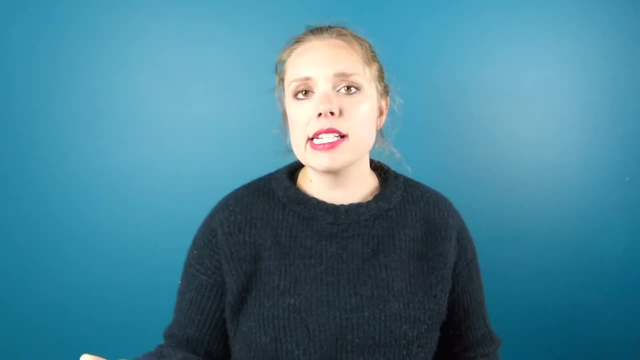 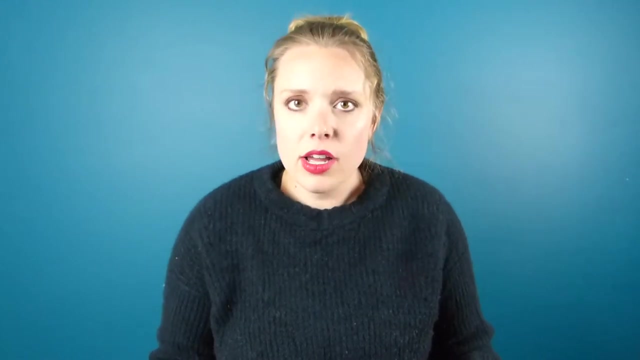 so that's something for you to maybe keep in mind down the road. but just as you're beginning to learn how to portion out your meals, it's not quite as important right now. so in my opinion, it's more important in the beginning of your weight loss program and just when all of this is feeling. 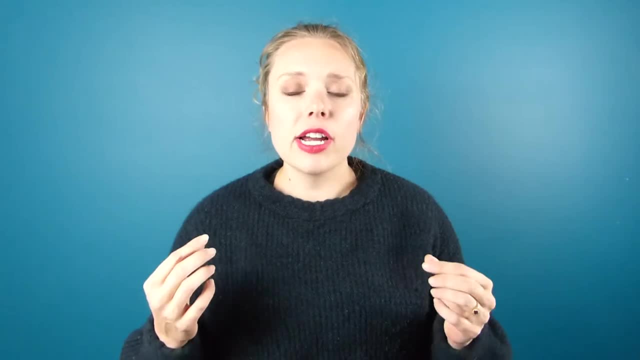 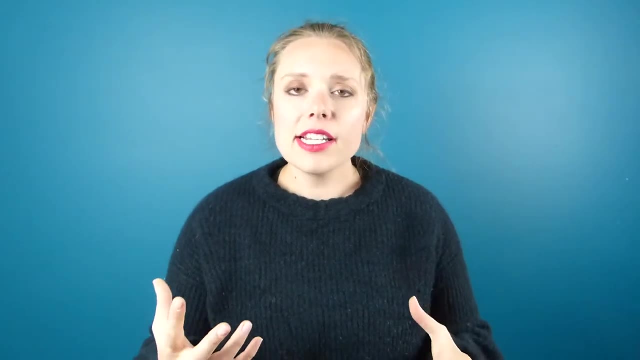 really new to you, um, to focus more on, like, creating meals out of whole foods that you're going to be out of, whole foods that have balanced portion sizes for you as an individual, And then, as you get more familiar with this process, then you can start to make note of things like: well, do I feel? better when I eat more carbohydrates and lower fat meals? Or do I feel better and more satiated when I eat like higher fat protein sources and oils and like keep the carbs lower? Everyone's a little bit different there, but I think once you've learned how to balance your meals in these 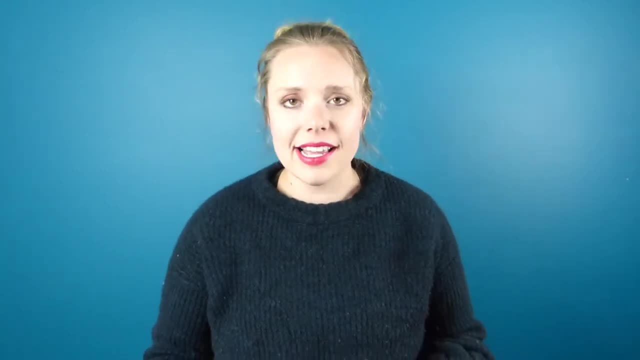 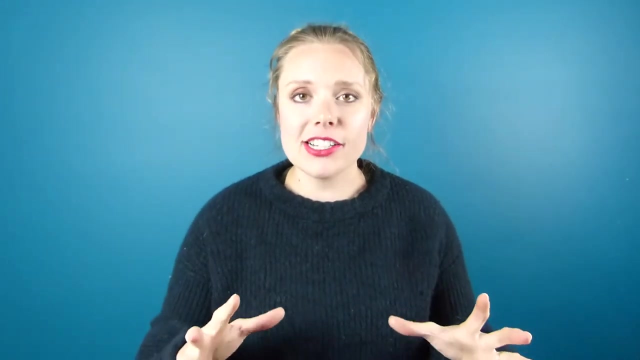 proportions. then you can start to pay attention to more things like that. You can also use this process while you're eating out at a restaurant, which I know might sound like it's really obnoxious to be like putting food in your hands when you're out to eat. You don't have to be that weird about. 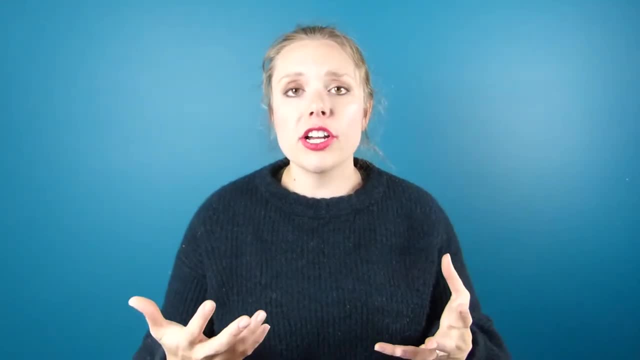 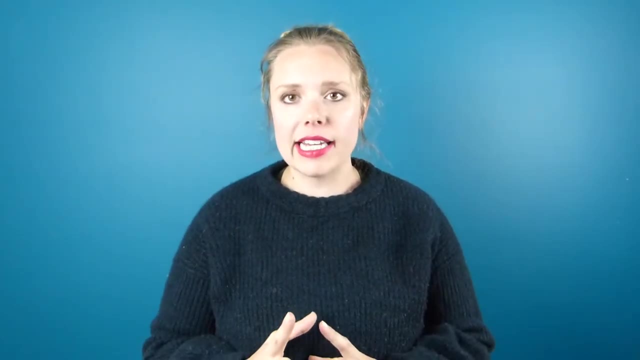 it Again, like the more that you do this, the more that you're going to be able to just eye things out by looking at it. But as you go, remember to keep it honest and not try to like expand the size of your hand, right?